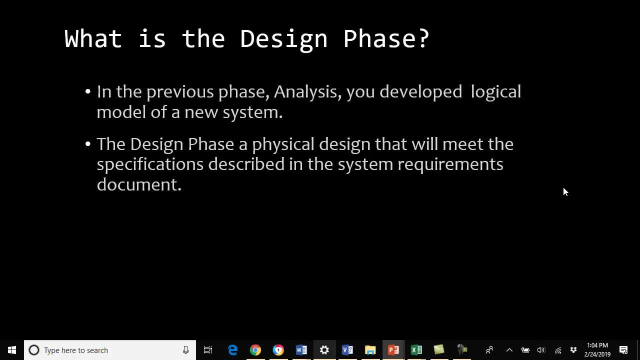 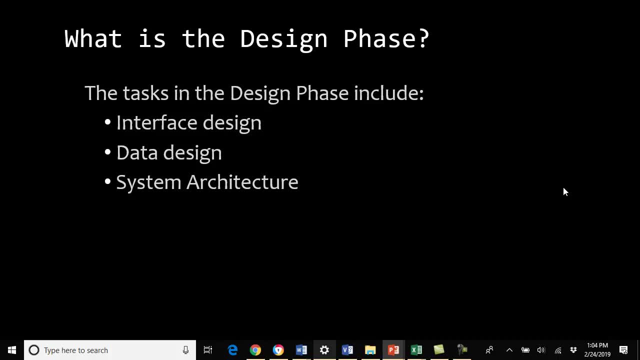 Now we're starting to get into the point of now doing the physical design and then we'll finally do the physical implementation in the development phase. What's this phase include? You know it can include all kinds of things, but based upon some of the literature we're using in this course, it really kind of goes down to these three pieces: the interface design, the data design and the system architecture. 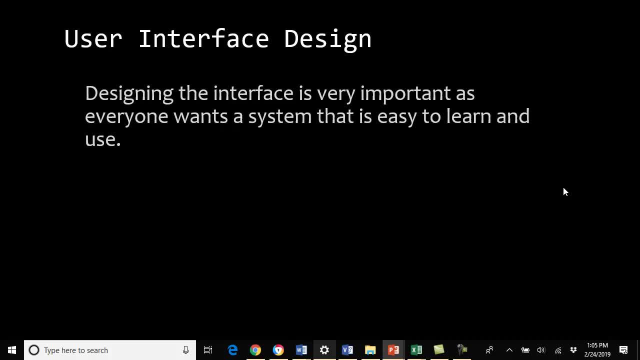 Okay With the design in the inner. So if you look at the interface design, the interface design is now exactly that. the interface design is a is very important. Everybody wants a system that it's easy to learn. We know that Okay. 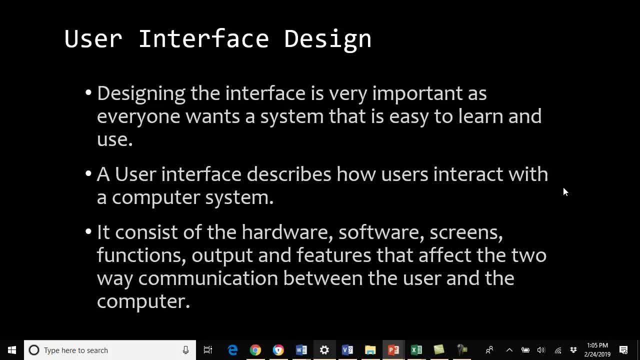 Designing the interface is very important, Easy to learn, use the user. The user interface describes how the user interacts with the computer system, Because this is the hardware software: screens, functions, outputs and features that affect the two way communication Between between the user and the computer. So let's look at that one more time. It's the hardware software. 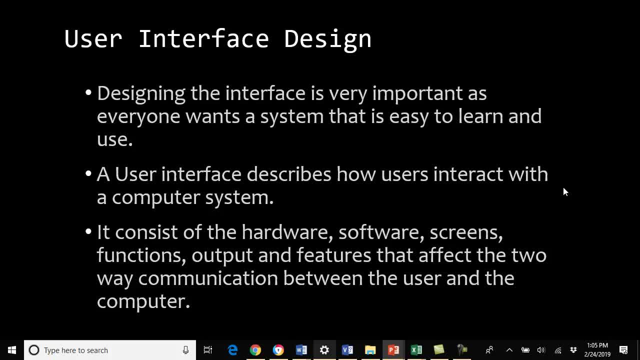 screens, functions, outputs and features that affect the two-way communication between the user and the computer. This can consist of, obviously, the forms, the screens, the GUIs, all based on about the same thing: The output from the output coming to these type of mechanisms, these forms. 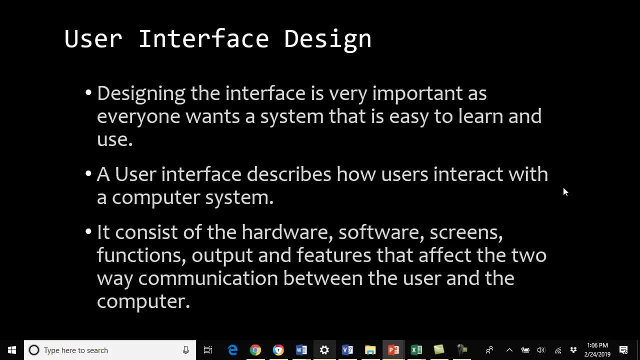 and these GUIs all the way to actual hard type reports, meaning paper reports that might actually go to the user also. This is the process of ensuring that all of this looks good. Once again, you're designing it out that your user says: this is exactly what I want. 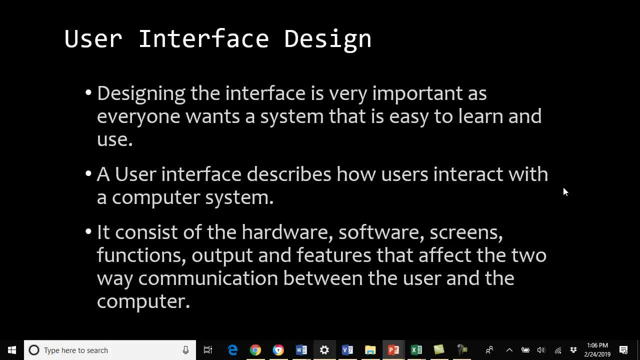 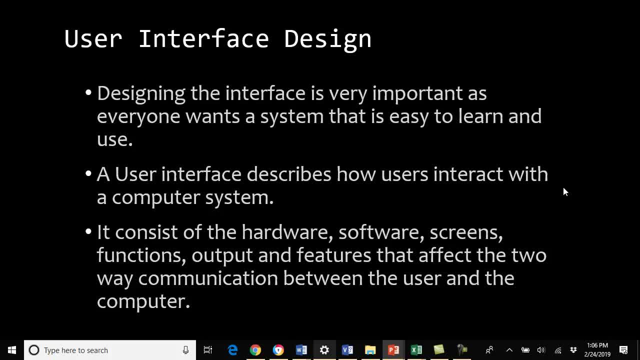 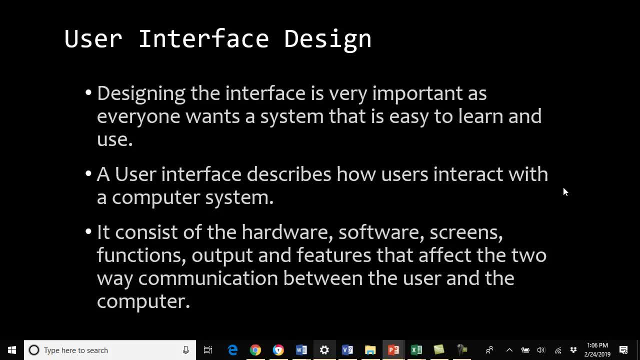 need this and I don't need that. That really starts helping us narrow down the scope a little bit more on exactly what the finished product is going to look like. If we didn't design this. we just went from specifications- basically the requirements- right to developments. 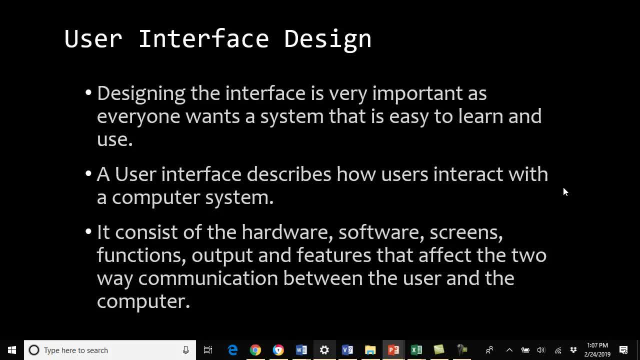 When we show them after all the development, they could look at this and say: that's not what I want. Next thing: you know we have just written a bunch of code for something they may not have needed, or we may have written code that is not giving them exactly what they want. Now we've got. 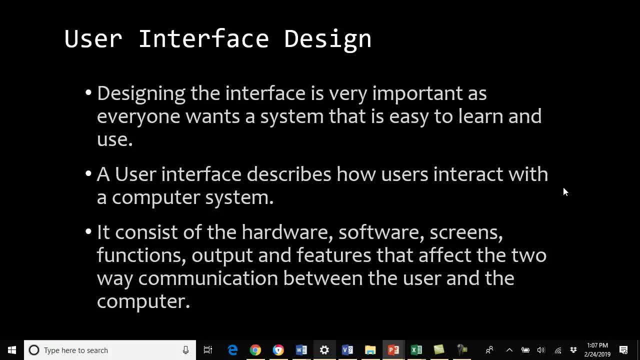 to redo a bunch of stuff. Who pays for that? The user doesn't like repaying for things, So this design process allows us to sit back and make sure we paint these pictures. It doesn't take much time to do this kind of stuff, Matter of fact, very little time in today's world with our technologies. 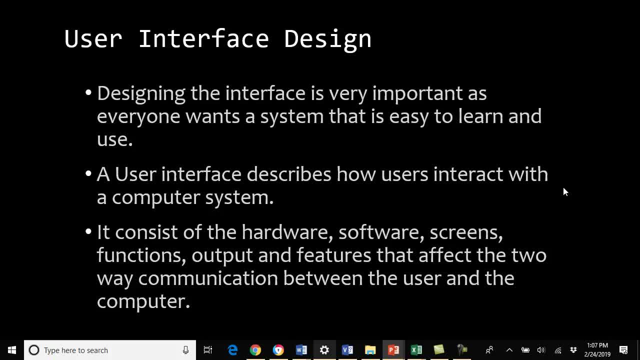 we have to paint these pictures, We have to paint these pictures, We have to paint these pictures. We have to paint a picture very quickly with Visual Studio and so on, to ensure that what they're thinking and what we're thinking coincide. That's what this is all about. A good design depends on. 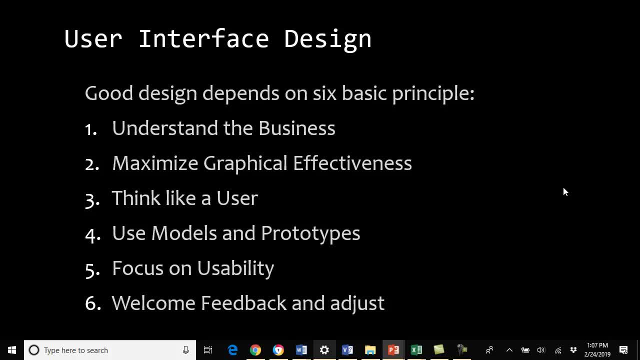 six basic principles: The understanding of the business that we're actually working for. They maximize the graphical effectiveness- We talk about this in many of our classes- Utilizing the controls on forms and so on that people are actually used to. If I were to dissect a page in order to create transitions, it would take two minutes. 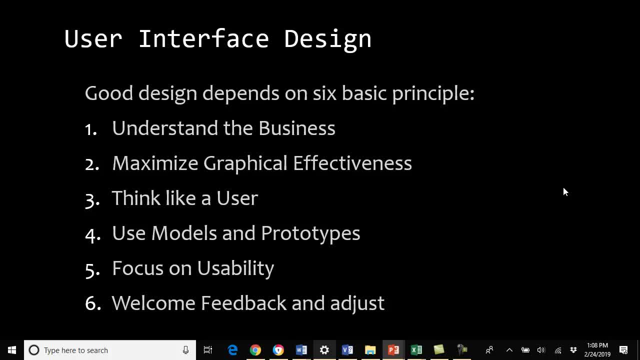 It would take about eight minutes for each line of graphic art to be reproduced as it was discussed. So it's time to think outside the box. Ahh, why you'd think outside the box and coloring those files in various languages? How do you think some of those writers have adapted that to the 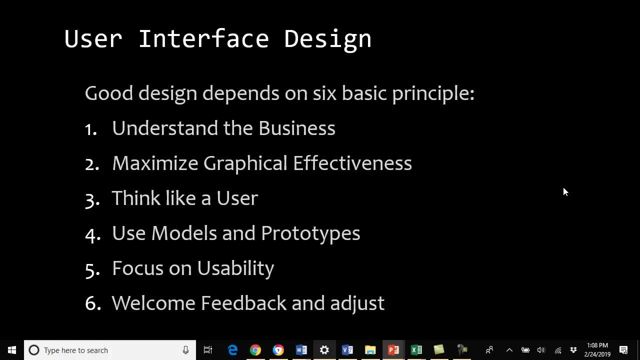 way you see it, and are they going to do which way in the format? We want to start thinking outside the box. so three elements that would get a kind of connection to the whole thing. Let's say the person is looking at a screenshot or something that 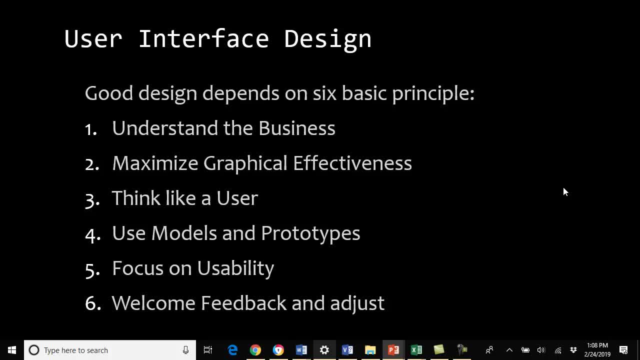 says: we're actually in custom language programming. we want to look at that projection or text. do we want to useこと so we could interpret it in that way? How does that work? If this doesn't work, how did you get an opportunity of sort of career, hoping to create something? Playages would do that. 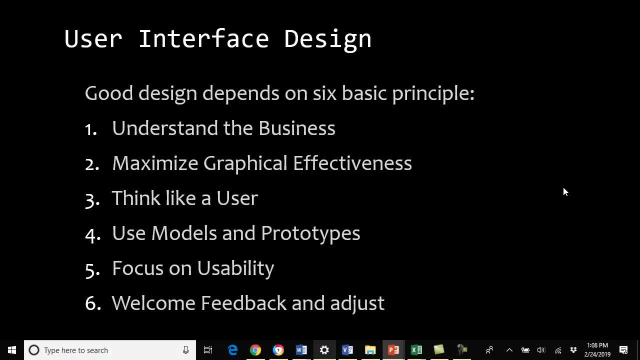 Building a storyboard is a great way of going through it. I have done things where I just start building screens out again using things like Illustrator or Visual Studio, and then taking them to my user to sit back and say: now, when you go here, you're going to click on this and do this. 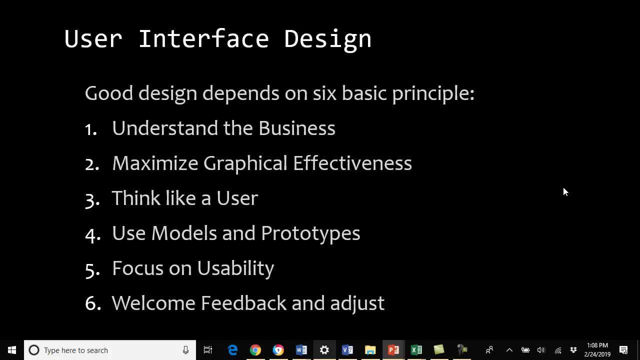 When you do this, it will go to here. When you do this, it will go to here. The whole idea is a storyboard out. I don't put any code behind it because, once again, I want to make sure what I'm doing is correct. 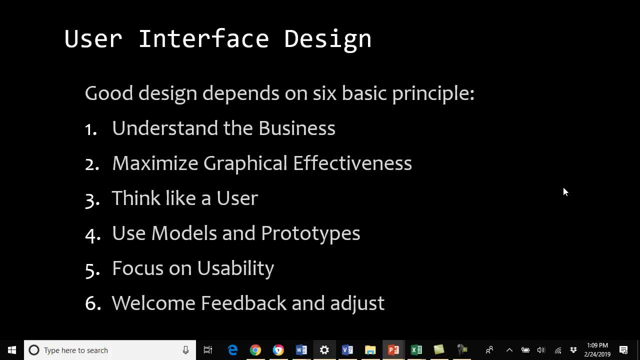 so I don't want to spend a lot of time coding anything until I know. this is what they're looking for. user-wise, interface-wise. We want to focus on usability. There's whole courses out there on human-computer interaction. that talks about how a human looks at a computer screen. 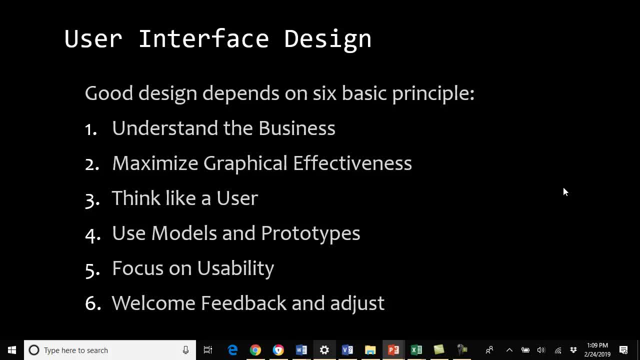 and how they anticipate interacting with that computer screen. With that said, we don't offer those courses right now in our curriculum, but there is whole courses out there and there's a whole psychology out there. We want to make sure we're building an interface that promotes interaction with its users. 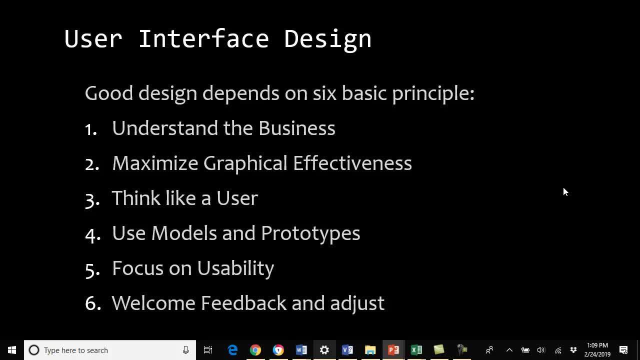 Also, whatever we do, we want to welcome the feedback and we want to adjust. during this phase, It's very important: Tell us what you like, Tell us what you don't like. Have people analyze it. If possible, have people who understand human-computer interaction analyze it. 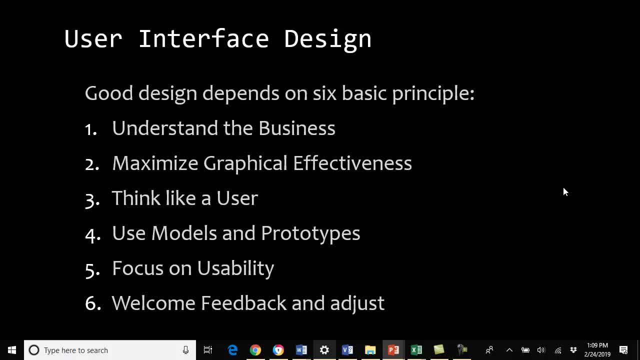 Make sure it's right. That's what you want to do. You want to welcome the feedback. You want to throw something out there, have people respond to it, modify it, throw it out again until finally everybody says that's what I want. 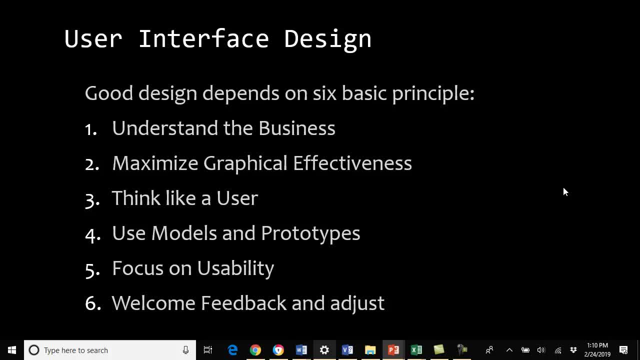 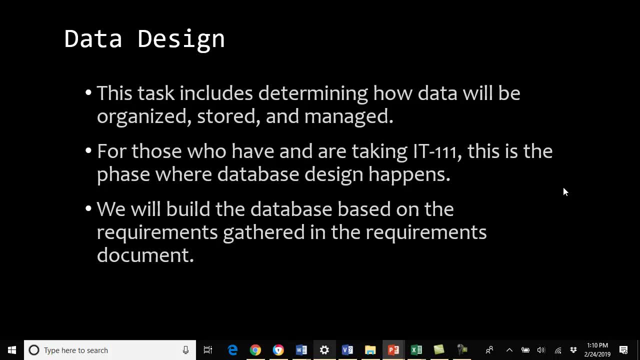 Again, this doesn't have to take a long piece of time at all. It can go very, very quickly, All right. The other piece of design phase is the data design For people who have taken our database classes here at Cincinnati State for the most part. 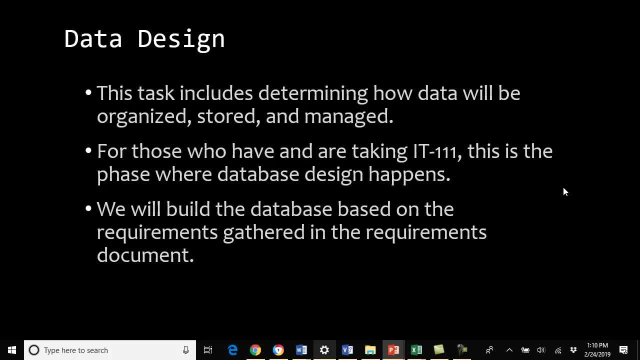 we're starting now with the whole idea of design based upon the requirements. Well, where do those requirements come from? Well, I'm kind of hoping if you have taken this IT111 already or you're in the process of taking IT111, it makes sense that you're seeing that it comes from the requirements of the requirements phase. 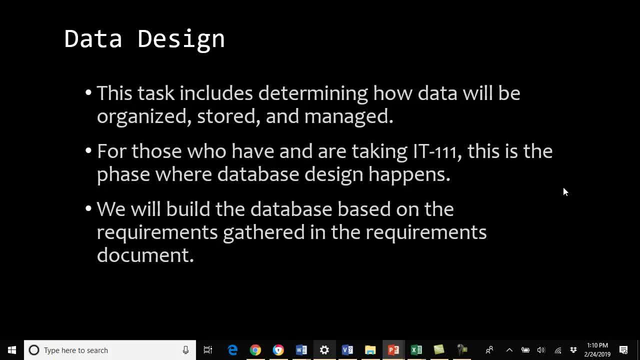 of the system development lifecycle. So, based upon that, that's what we're going to be doing. So the goal of the data design includes determining how the data will be organized, stored and managed. We're talking about the data that's going to be organized, stored and managed. 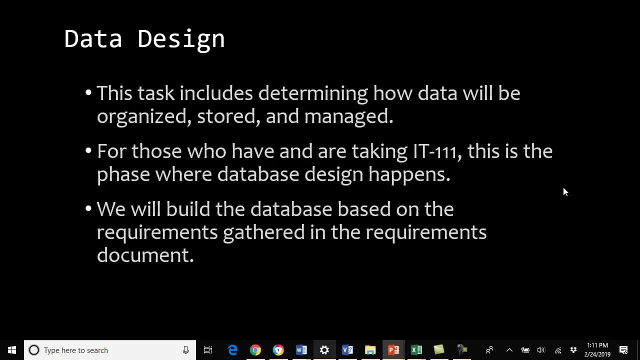 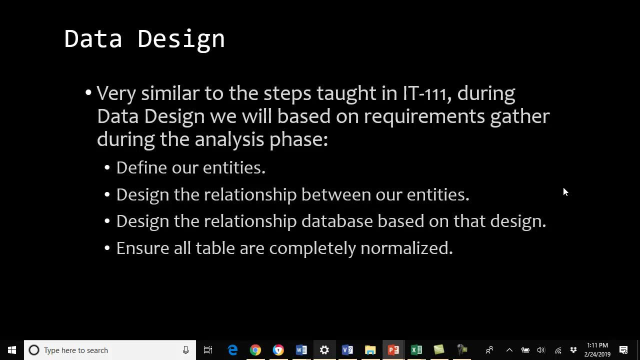 We're talking about in a database of some sort, Cincinnati State. we work with SQL Server, a little bit with MySQL, those type of databases. We're going to build them based upon the requirements that we actually had gathered, Very similar to what we did in IT111, we'll go through and understand the requirements. 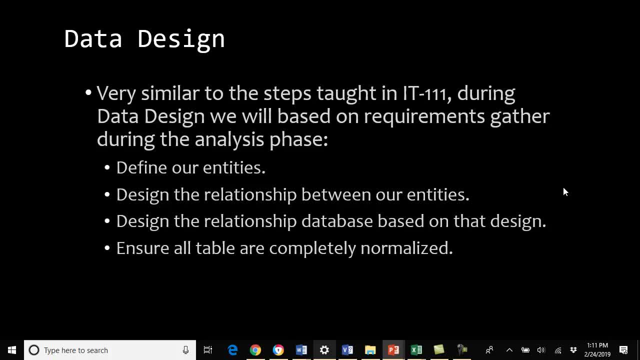 And, based upon those requirements, understand our entities, the relationships between the entities. We're going to design the relationship database based upon that design And we're going to build them based upon the requirements that we actually had gathered And we're going to ensure that it's completely normalized. 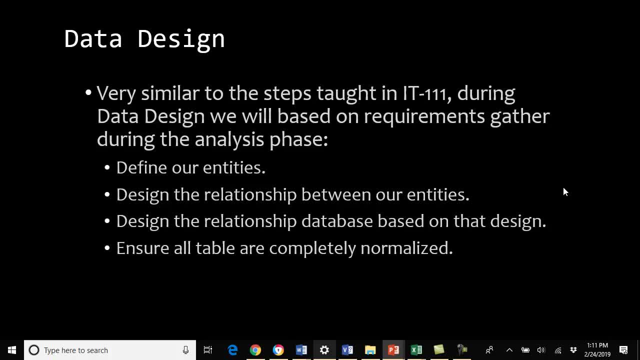 Once again, if you haven't taken IT111, that's what you're going to be doing in it. If you have taken 111, I'm hoping by listening to this you start realizing where those initial requirements come from, And again from the requirements phase of the SDLC. 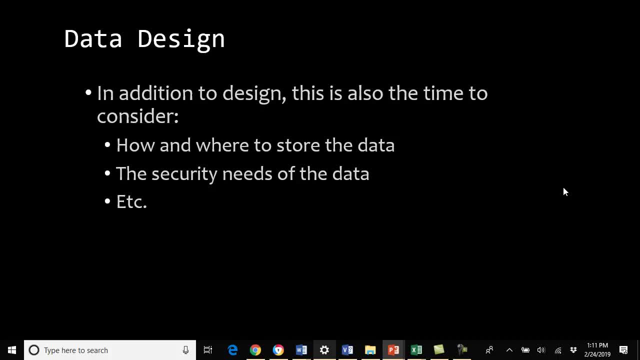 In addition to the design, there's also time to consider how and where the data is going to be stored, the security needs of the data, et cetera. We need to make sure we understand What's the term I'm looking for. 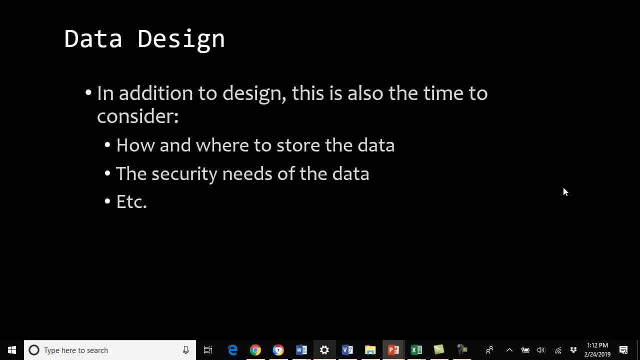 The security of the data, how important it is, who can get to it, who should not see it, those types of things. Based upon that, we're going to start working with the architecture piece of this to ensure that the data is 100% secured all the way through. 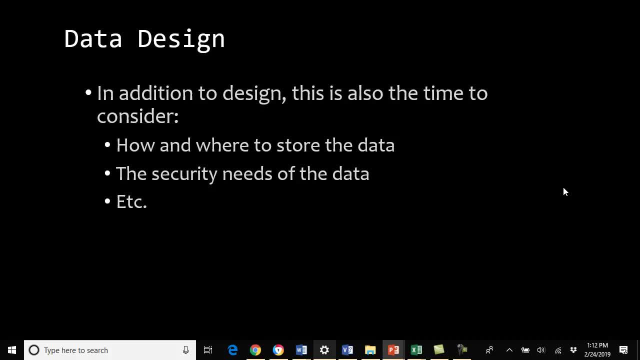 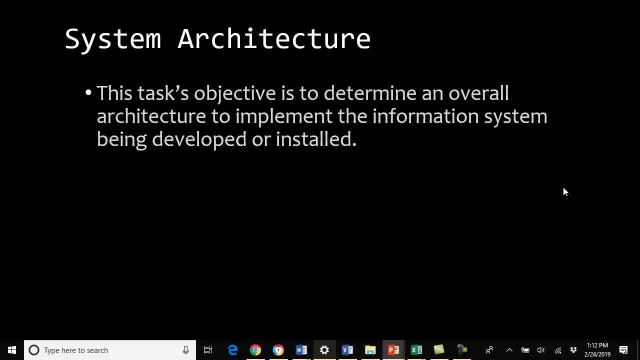 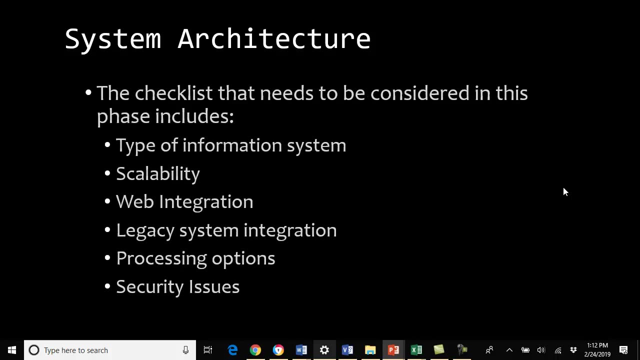 I hope that makes sense. So you need to understand that as you kind of go through it. Okay, The system architecture: as I mentioned before, this task objective is to determine an overall architecture to implement the information system being developed or installed. So when we're talking about the architecture, we're basically talking about the computers needed. 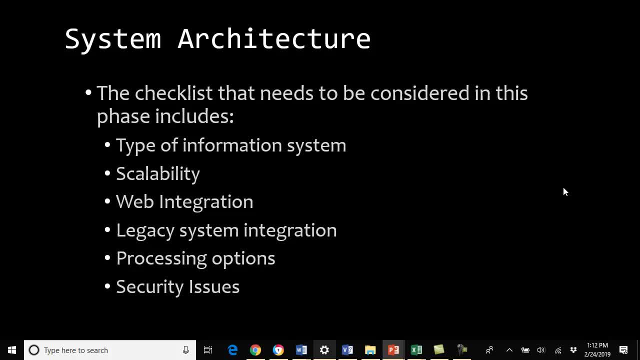 the network needed, how it's going to be utilized, where we're going to implement this new system. what kind of, let's say, computer or server or so on, are the system going to be put on? In a lot of cases, there's so much that goes into this piece. 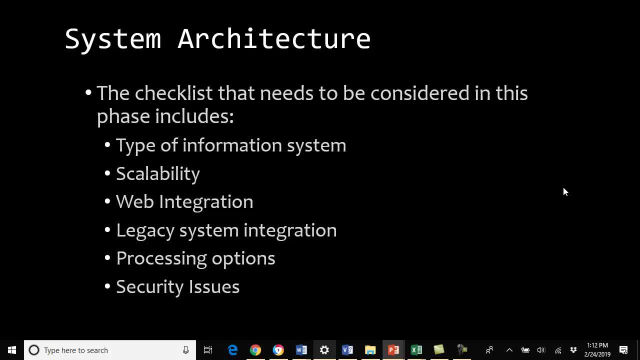 We don't talk about it much- And Our current curriculum, but this is where all the networking and everything else comes into play, Based upon what I have done and throughout my career. we have specialists who deal with this architecture. I give them the requirements based upon what my database is, the security needs of my database. 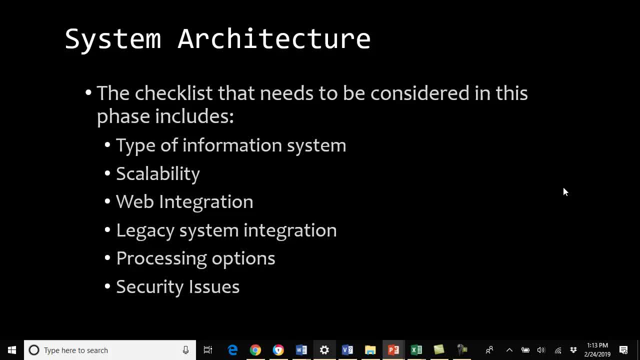 the access needs I have to my database, what my application is going to be in regards to a web-based application or a Windows-based application or so on, And then, based upon that, we'll sit down and draw a plan on how this thing needs to be implemented. 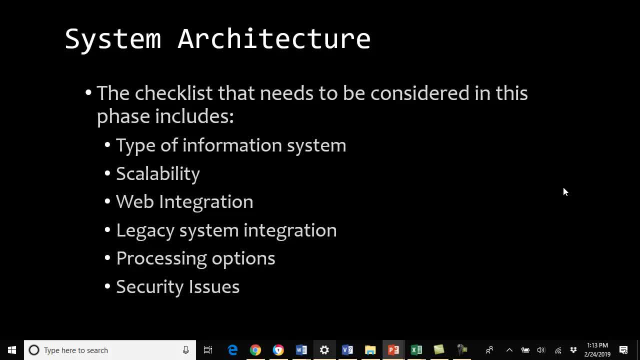 It could be as simple as you know: just a server, a web server, with everything on it. or it could be as complex as putting it behind several firewalls and making sure the security is there and only certain people can get to it. 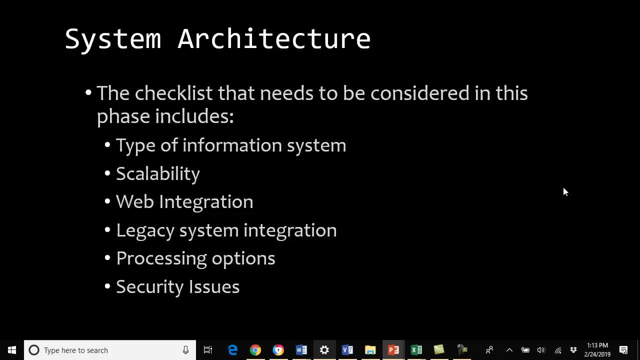 So in this case, here, what we want to consider is the type of information system, the scalability. How is this thing going to grow? Is it going to grow by crazy, or is it going to be maintained with its certain uh size right now? 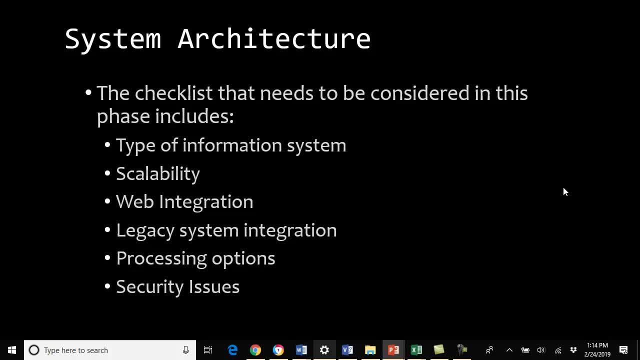 How is it going to integrate with the web? Does it need to integrate with anything else outside of its platforms or its actual application in regards to the web? This whole piece about legacy systems: you might not know what those mean. Those are old systems to a company, systems that have been developed, I don't know, 10,, 15,, 20,, 30,, 40,, 50 years ago. 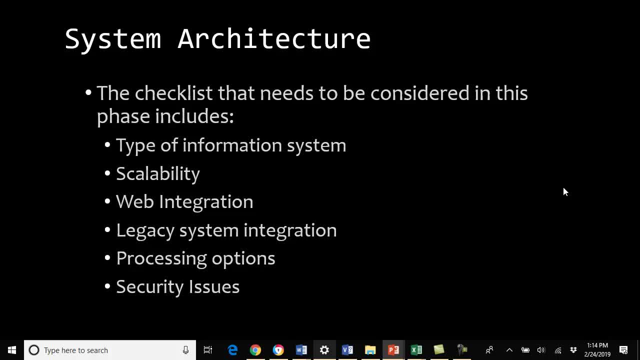 but they're still using them And, trust me, they're still out there. How can we integrate with those if our system needs to integrate with it, Our processing options And, again, our security issues actually go through it. This all plays in the part of system architecture. 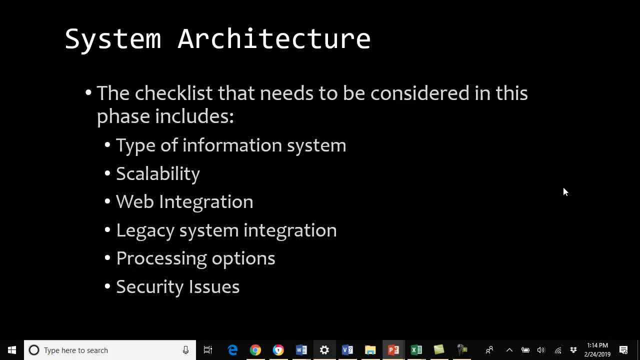 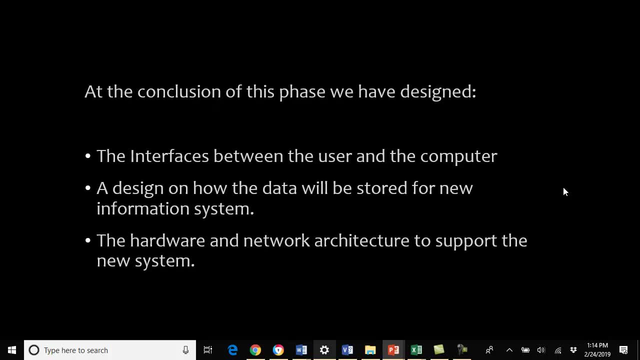 If you go look at the book that we recommend you look at it, you read a review, you'll see different types of scenarios when it comes to architecture. that can be considered. All right. Again, this design, kind of quickly going through, it is not overly complex. 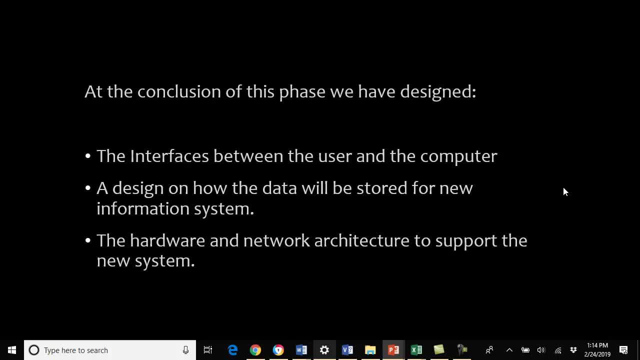 Again, I don't think any of this is overly complex, but at the conclusion of this phase we have designed. The interfaces between the user and the computer are a design on how the data would be stored for a new information system and the hardware and network architecture to support the new system. 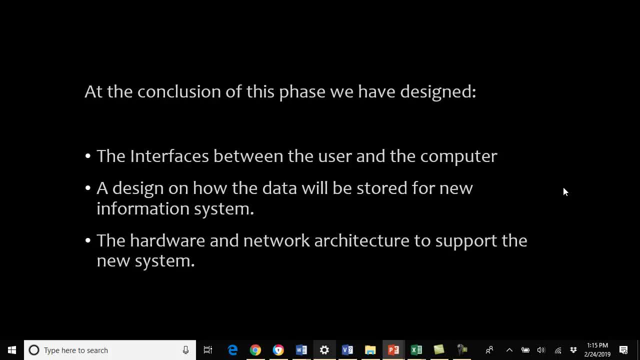 That's what this thing's all about. Hopefully, you kind of see the progression here. You have an idea, we got the requirements and now we have it all designed out. The goal would be, as you would review this whole design, especially the interfaces and so on, with your users. 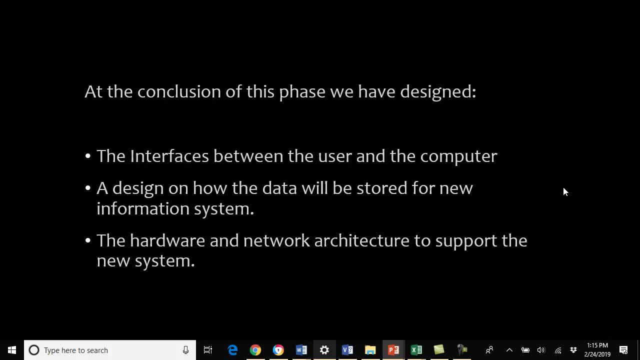 Pretty much all of it. They're not going to understand the database as much if you start talking databases to you user but in regards to the interfaces and then pretty much giving them an idea of how you know that's going to be supported. architecturally wise is something that you